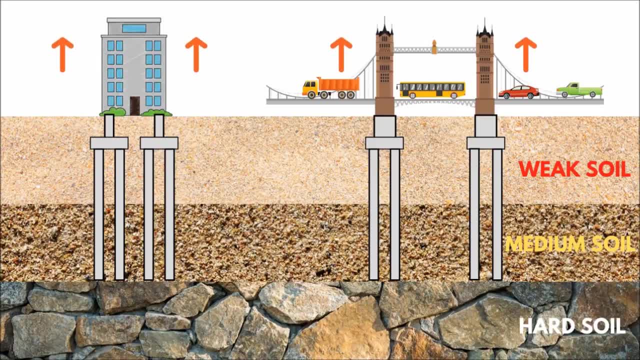 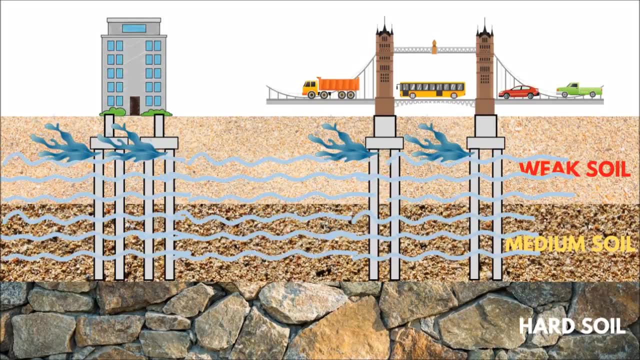 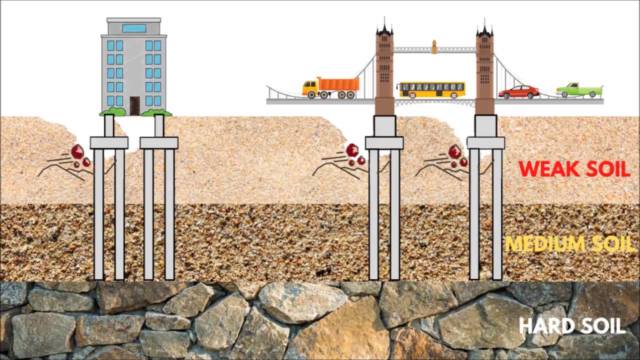 uplift forces created due to water table rise or any other cause will affect the foundation badly. Pile foundation is the solution here. Pile foundation is necessary for those areas where the structure surrounding has chances to be damaged. Pile foundation is the solution here. Pile foundation is used for soil erosion and scouring. 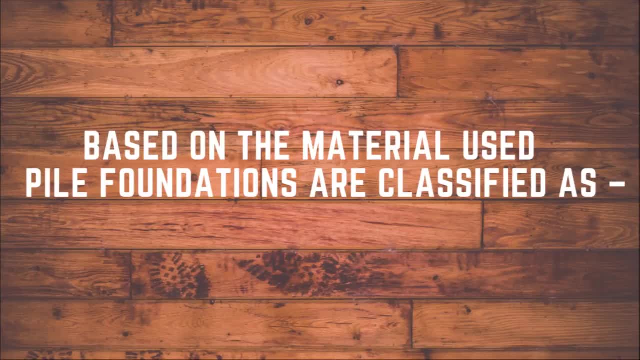 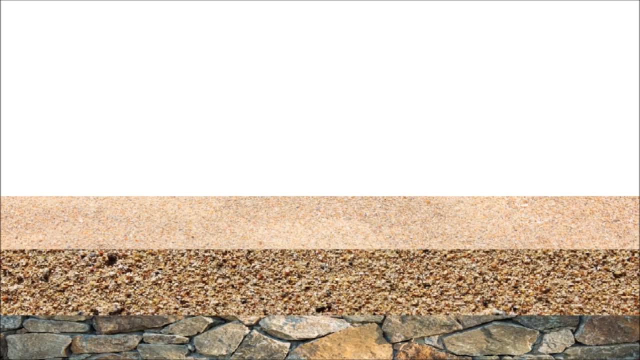 Based on the material used, pile foundations are classified as timber piles, steel piles, concrete piles and composite piles. Types of Pile Foundations Based on Construction Method: Driven Pile Foundation. Driven pile foundations can be made from concrete, steel or timber. These piles are driven using. 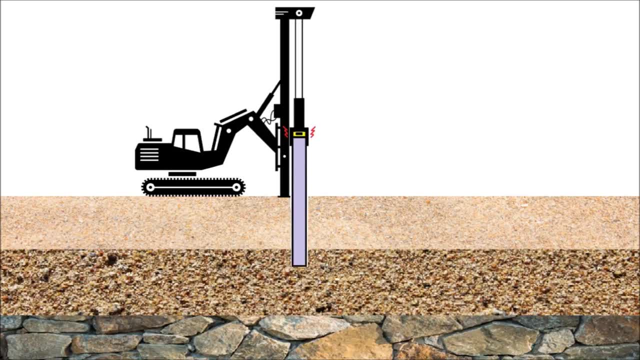 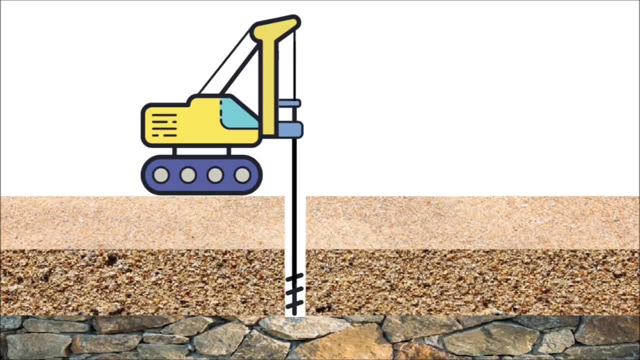 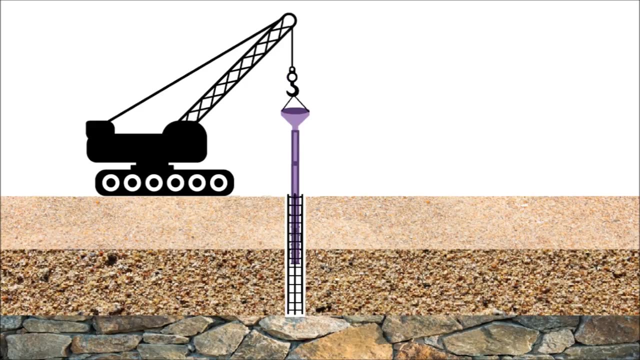 pile hammer by dropping weight or vibrating Board Pile Foundation. These piles are constructed by drilling holes in the ground up to the required depth, then inserting the reinforcements as per drawing and the trimmy pipes as per requirement, and finally filling the hole with the fresh concrete. 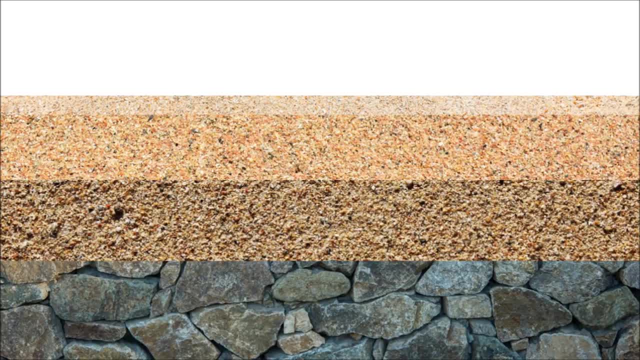 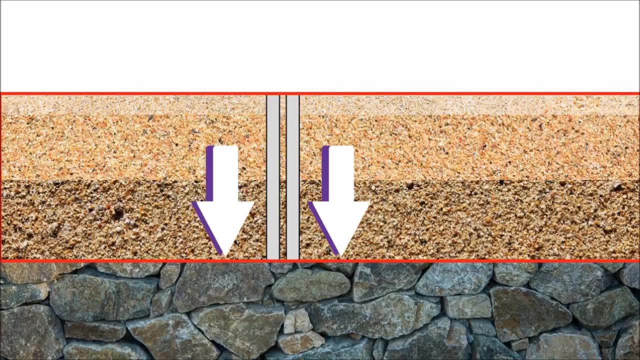 Types of Pile Foundations Based on Structural Behaviour: End-Bearing Piles. In end-bearing piles, the load is transferred through weak soil to the strong soil. The bottom end of the pile rests on the layer of hard soil or rock. As a result, the pile acts as a column and safely transfers the superstructure loads. 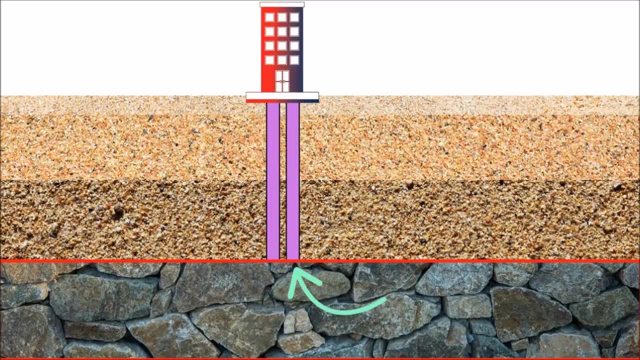 to the strong layer. The capacity of end-bearing pile can be calculated by multiplying the cross-sectional area of the end of the pile. The end-bearing pile is the area of the end of the pile. The end-bearing pile can be calculated by multiplying the cross-sectional area of the. 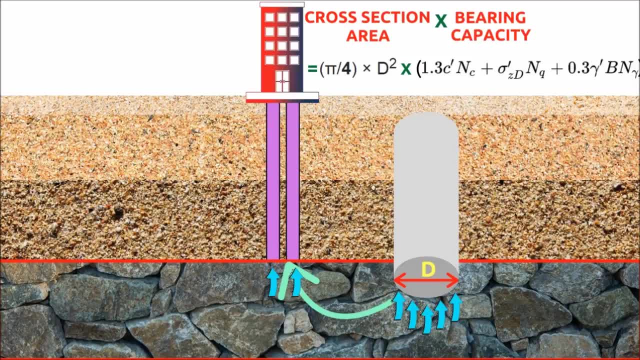 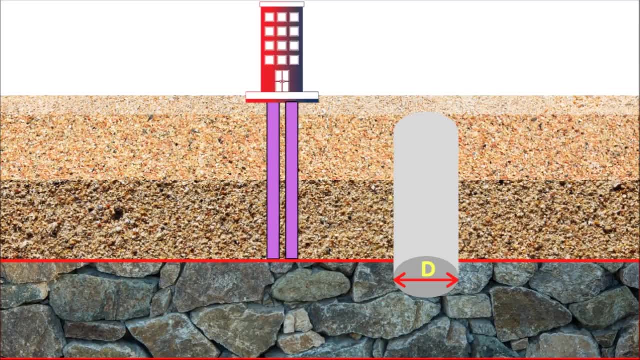 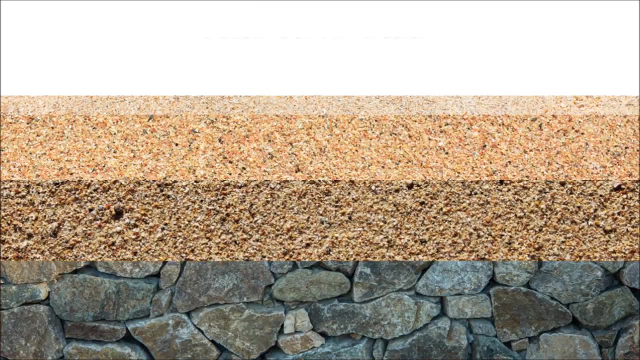 end of the pile, The heavy soil and the bearing capacity of the hard soil in which the pile is resting, with considering a reasonable factor of safety. The total capacity of end-bearing pile can increase by increasing the number of piles and pile diameter: Friction Piles When the hard strata exist in large depths. 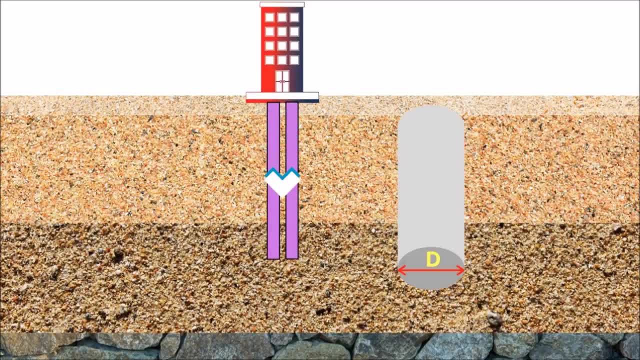 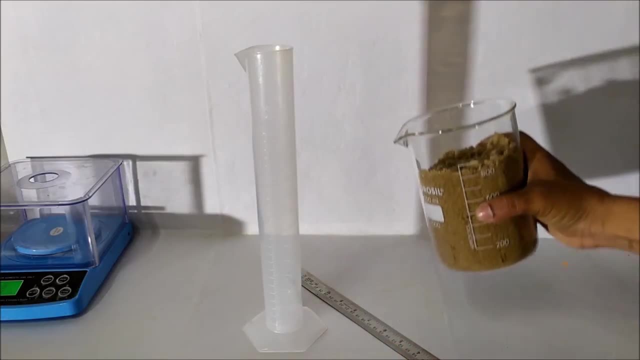 friction piles are used. It transfers the load from the structure to the soil by frictional force between the structure and clay soil surface of the pile and the soil surrounding the pile. Here this is the soil and the scale is acting like a friction pile.